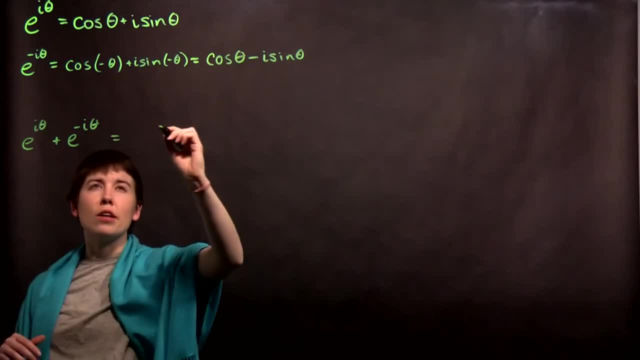 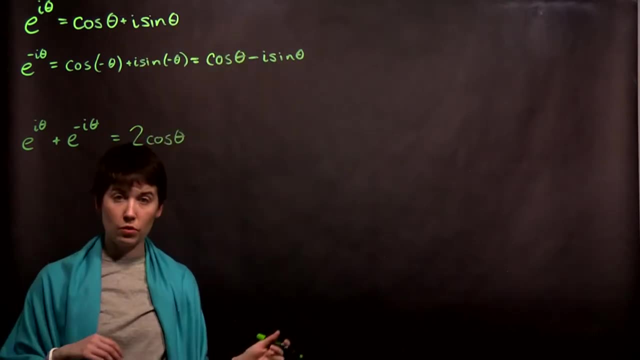 going to have cosine theta plus cosine theta, which is 2 cosine theta, and then I have i sine theta minus i sine theta, which is 0. There we go. The way you're going to often see this written is that cosine theta is the same as cosine theta and that cosine theta 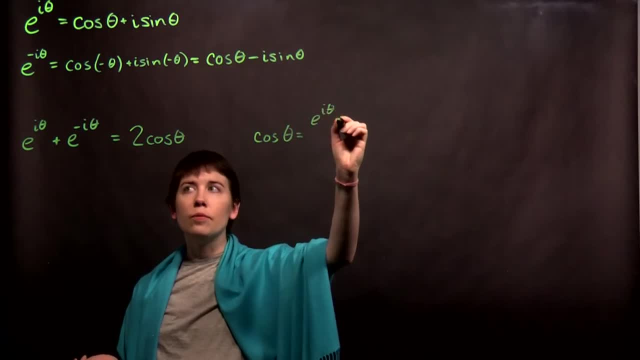 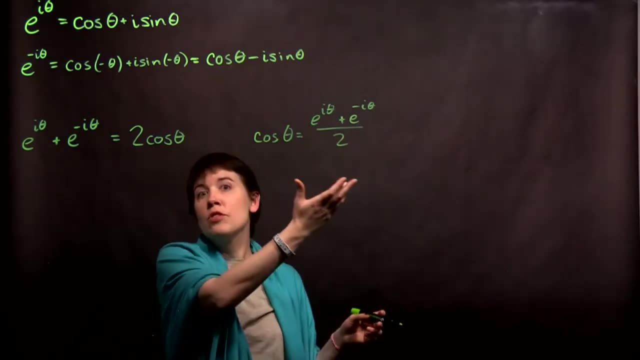 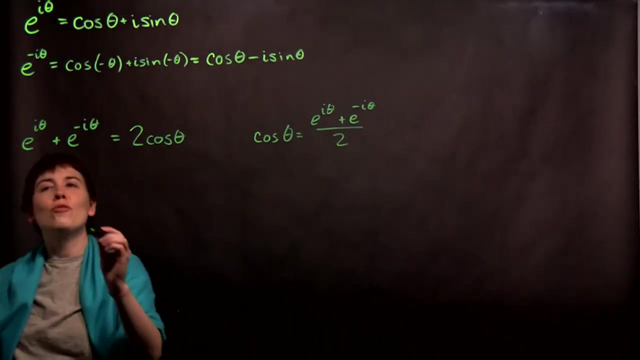 is the same as cosine theta, So that cosine theta is going to be e to the i theta plus e to the minus i theta over 2.. So that's a relation that you might have seen written somewhere in the back of a book, but you can get it just from knowing this. So if we subtract, 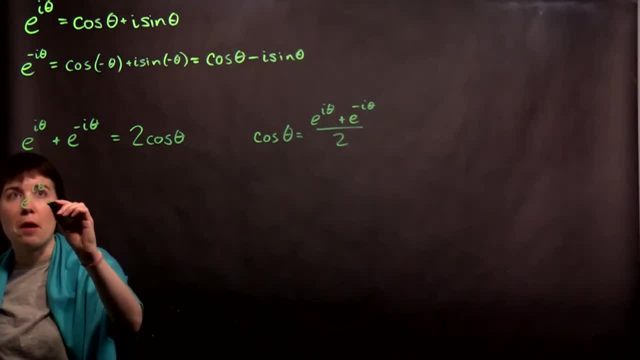 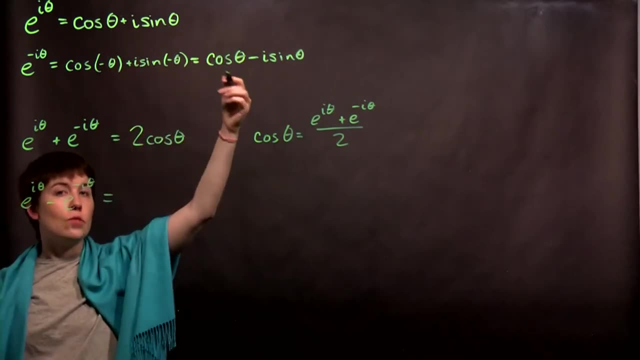 them, we'll get the other one. So e to the i theta minus e. so the negative i theta cosine minus cosine is 0.. And the reason why I'm kind of breaking it up that way is that this cosine term is real. 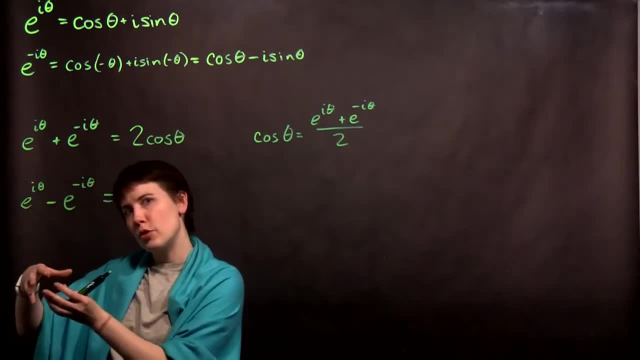 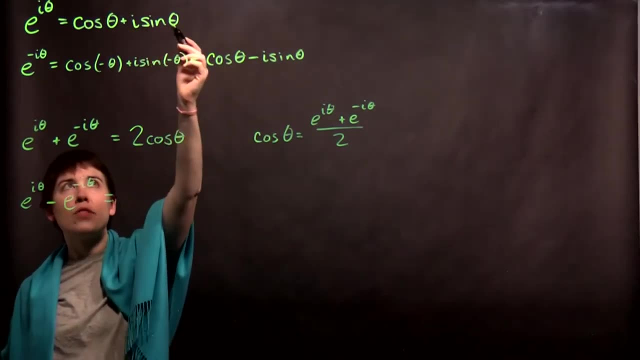 This sine term is imaginary. So you can kind of think about grouping your real terms together and grouping your imaginary terms together. So cosine minus cosine is 0. But then I have i sine theta, minus minus, i sine theta, So that's 2i sine theta. 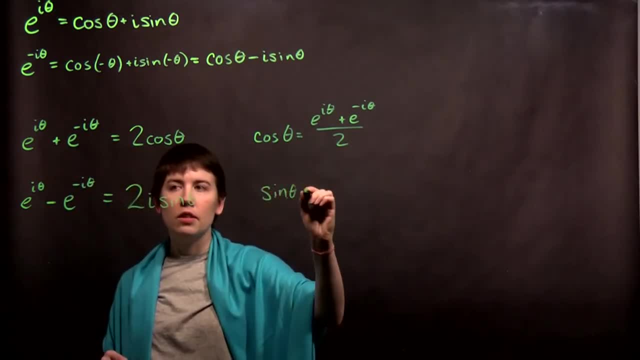 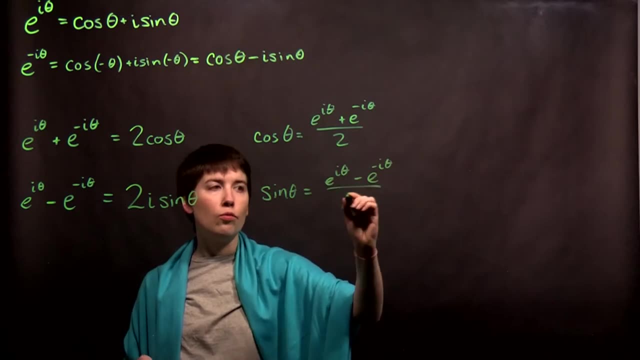 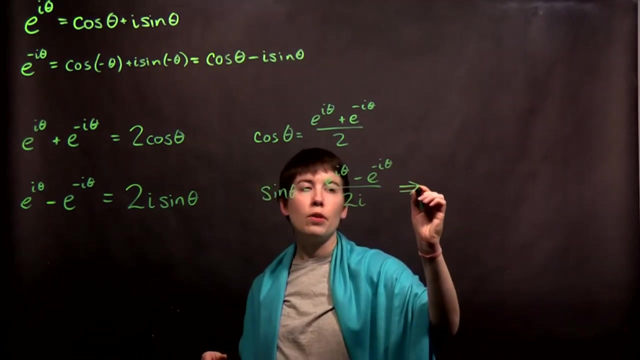 And so in that case I could say: sine theta is equal to e, to the i theta minus e, to the negative i theta over 2i. If you wanted to, we could rearrange this. We could, for instance, multiply both the top and the bottom by i. 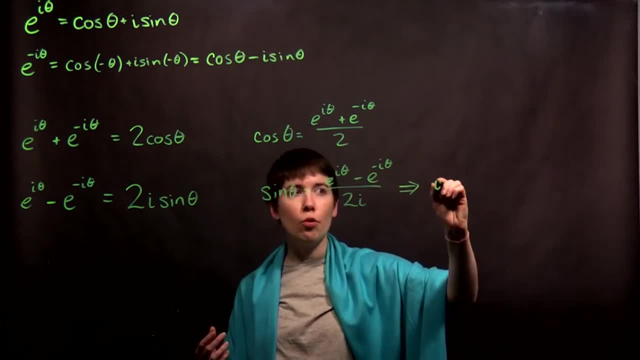 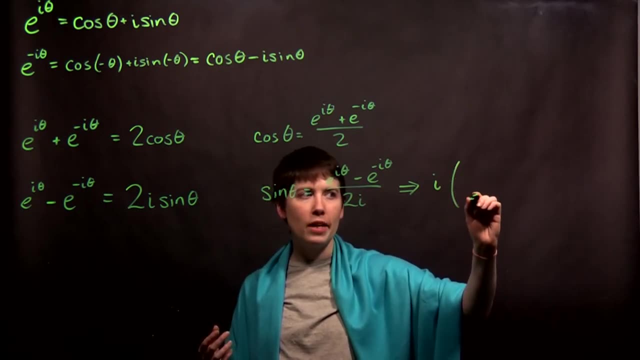 if you don't like i on the bottom. So that would give you an overall i, But because we've multiplied i on the bottom, that would actually give us negative 2.. So it's not really very nice to write it this way. 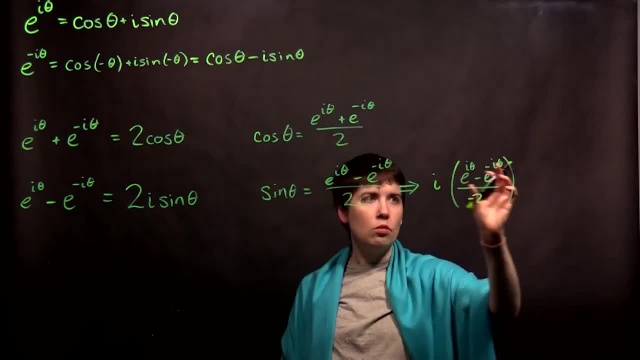 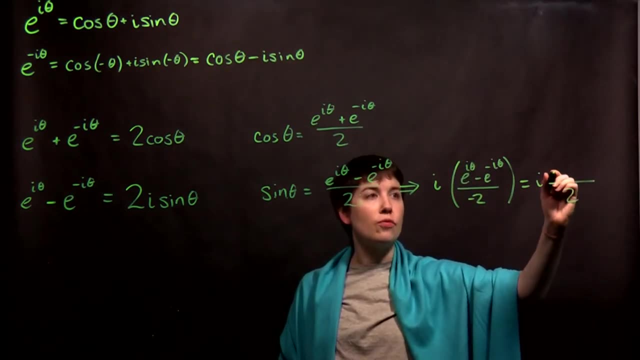 So what you could do instead is say, oh, we'll just flip that around, And so if you want to keep that, i separate and on top you would actually flip the signs here And this would become e to the negative i theta minus e to the i theta.